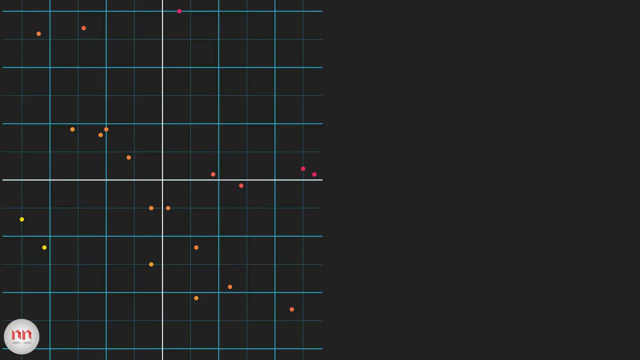 If you are familiar with linear regression, you can see that it's easily solvable by finding a best fit 2D line. that is a plane. But how can we solve such a regression problem using a decision tree? Well, the general concept is the same as the decision tree classifier. We recursively 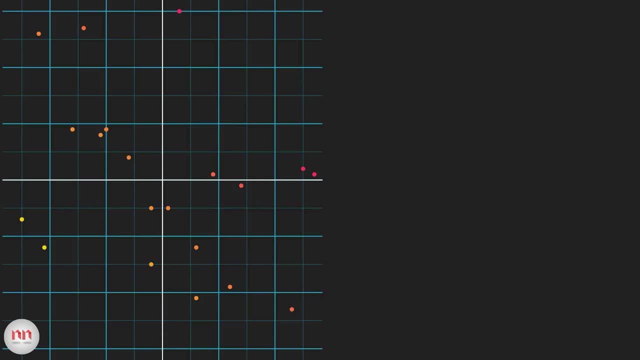 split the data using a binary tree until we are left with pure leaf nodes. There are just two differences: How we define impurity and how we make a prediction. For now, keep these two questions in the back of your mind. I will explain them later. 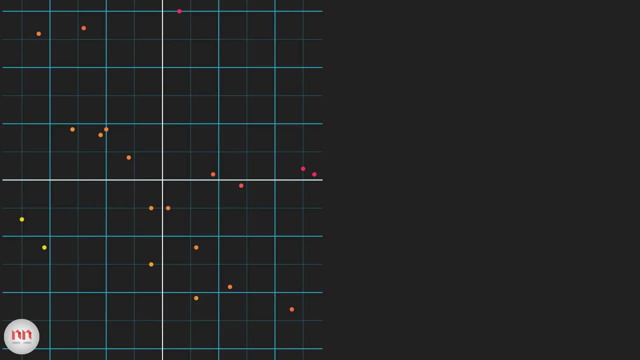 First, I want to show you the decision tree for this problem and how it splits the dataset. So here is our tree Focus on the root node. I am taking all the data points here. As you already know, now we are gonna split it based on the condition of the root node. The condition is: 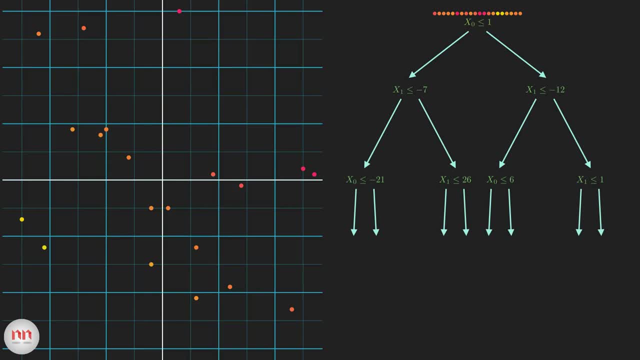 whether the x0 feature is less than or equal to 1.. In the plot the splitting condition looks like this vertical line. Every point that lies either left or on the line satisfies this condition. We will place those points in the left child And the points that 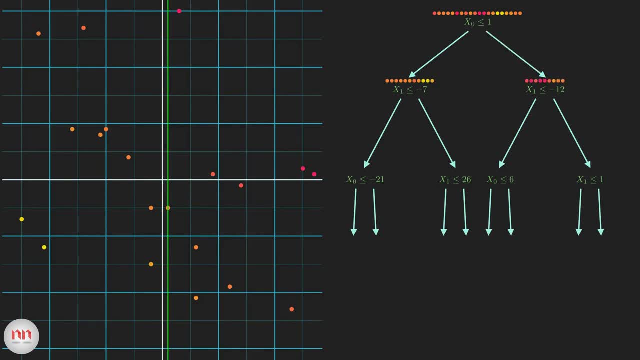 don't meet the condition will go to the right. After the first split only you can see the yellowish points are on the left and the reddish points are on the right. This shows that the impurity of the nodes are reducing. We are gonna follow this split. 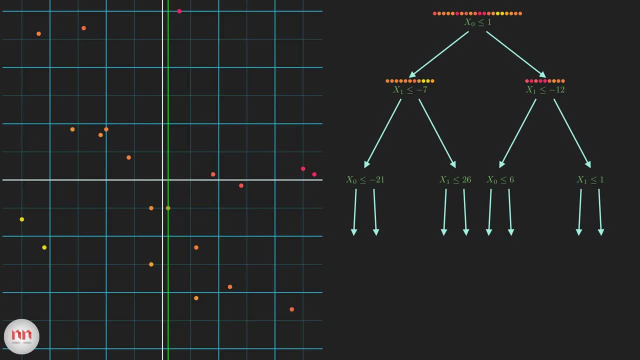 rule for all the remaining nodes. Let's turn on the autopilot. The next next step: we will split the distance between the nodes, and the nodes should be 0.. The right and left some points. Thezon's infectivity will be less than 1, the left and right will be 0.. 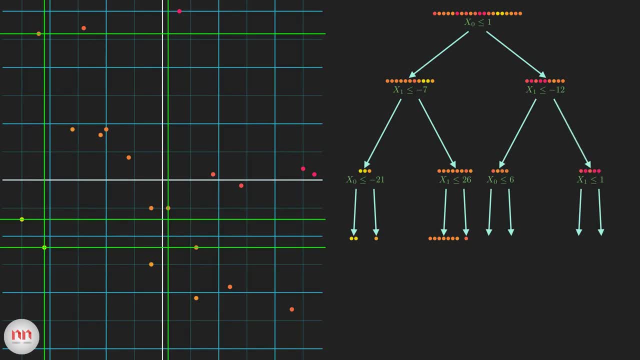 And the left and right will be 1.. The left and right is now 0, so the left and right will continue to be 0. So the live and the live are completely 0. So we can now put the node in the right place and the node can be cut off. 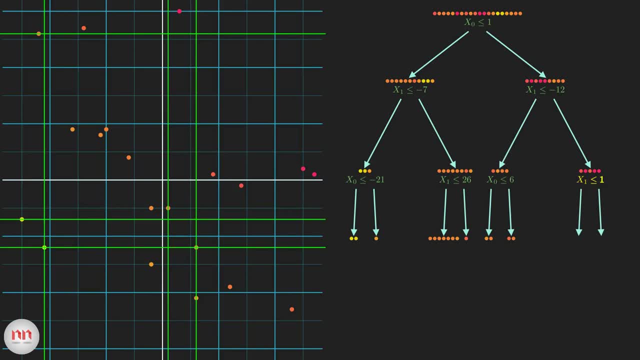 That's the first step. Let's cut it off. Okay, here's the complete regression tree with the proper splits. Now the question is how to predict the y-value of a new data point. Let's have a new point at. At first, we check if x0 is less than or equal to 1.. 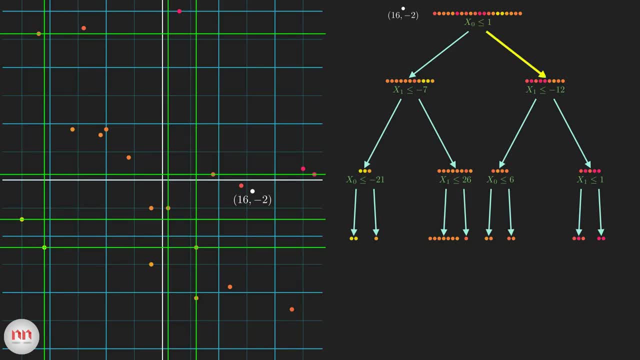 It doesn't satisfy this condition, So it goes to the right. Here also, the condition fails and we move to the right. Finally, this condition is true. hence we move to the left. So we arrive at a leaf node that contains only three data points. 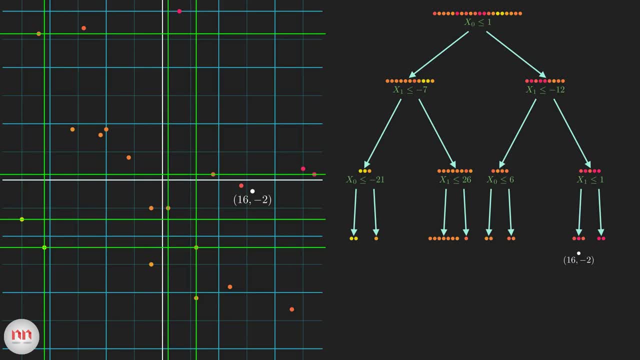 To predict the value of our new data point, we just need to find the average y-value of all the three data points present in this leaf node. Yes, it's that simple. The prediction turns out to be around 181.. By following the same method, we can predict the y-value of any point on this 2D plane. 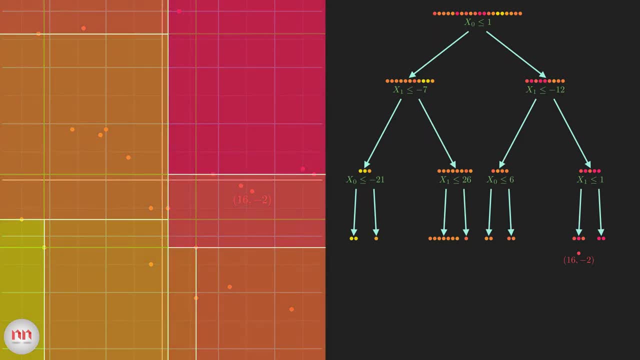 Let me show you how that looks like. The interesting thing is, even though it was a regression problem, still we end up dividing the feature space into several regions, which is very different from other regression techniques. Let's see: The color of a region tells you the predicted value of every single point in that region. 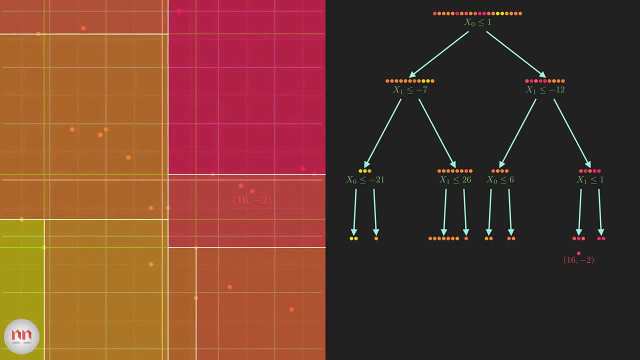 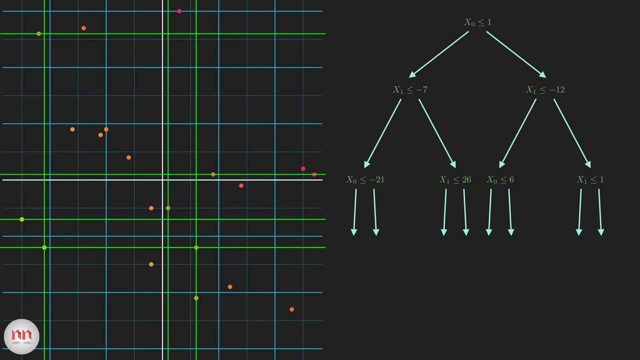 Okay, now comes the most important part: How do we split the dataset? Let's clear the clutter and focus on the root node. Here we will have the whole dataset And the task will be to find the best splitting condition, Just like my previous video. 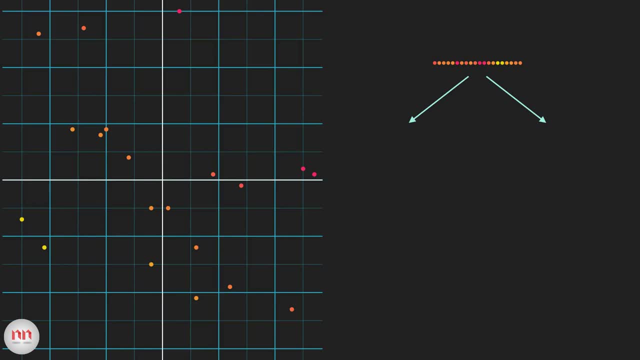 We will examine two candidate conditions. The first condition is x0 less than or equal to 1.. If we follow this condition, then the splits will look like this: Our second condition is x1 less than or equal to 2.. In this case, the division is like this: 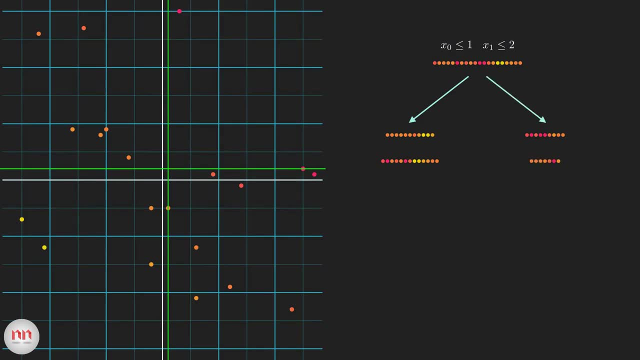 Don't forget that the points that satisfy the condition go to the left and the rest to the right. Now the question is: Which is a better split? To find this, we need to calculate which split is decreasing the impurity of the child nodes. 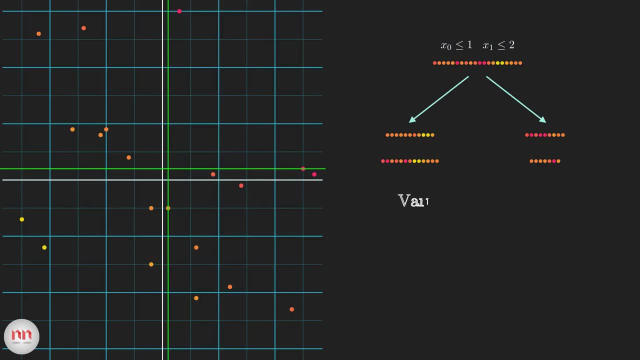 the most. For that we need to compute variance reduction. Yes, in the context of regression, we use variance as a measure of impurity, Just like we used entropy or Gini index in the classification problem. Focus on the complete dataset. 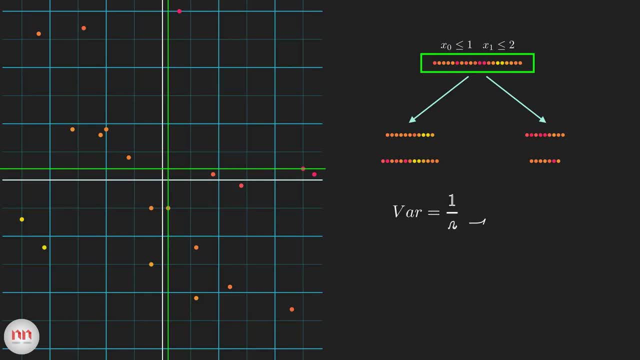 We are going to compute the variance of the whole dataset Using this formula. Remember, a higher value of variance means a higher impurity, So the variance at the root will turn out to be this: Similarly, let's compute the individual variance for all the divided datasets. 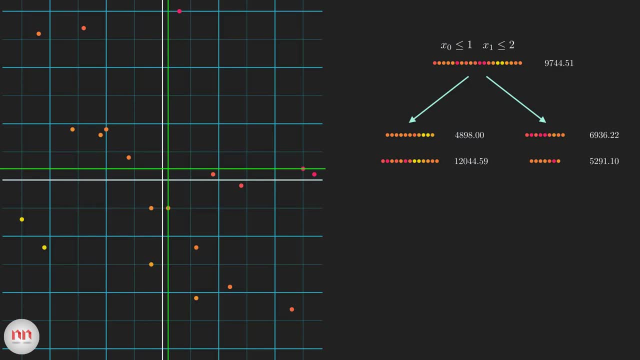 Ok, Now we need to compute the variance of the entire dataset. Ok, Now we need to compute the variance of the entire dataset. Ok, the variance reduction. For that, we just subtract the combined variance of the child nodes from the parent node. The weights are just the relative size of the child. with respect, 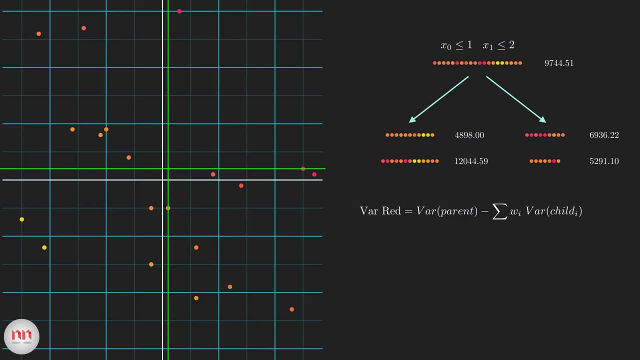 to the parent. Let's compute this for both the splits. Just look at this. The variance reduction for the first split is so much more than the second one, And it makes sense because in the first split there is a significant difference between the child nodes. The left one has more yellow points and the right one has more. 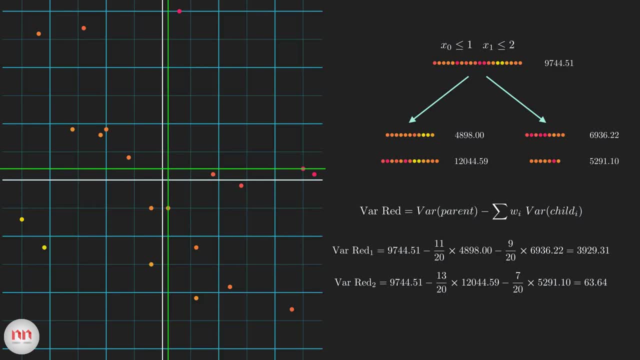 red points, But in the second split the red and yellow points are kind of mixed in both the nodes. This tells us that the first split can decrease the impurity much more than the second one. So finally we come to the conclusion that we should choose the first one. 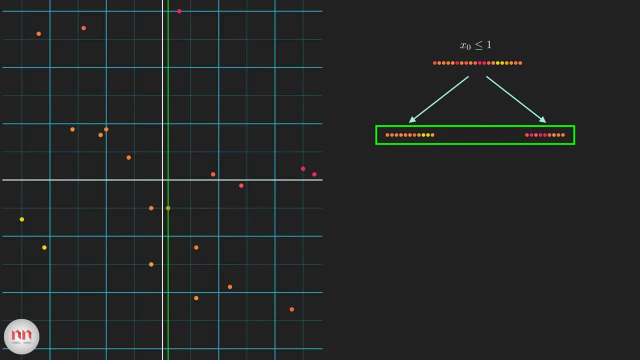 Here we only compared two splits. In reality, the model evaluates the variance reduction for every possible split and selects the best one. This process of selection happens recursively unless we have reached our desired depth. I hope now you have a very good understanding about decision tree regression. In the next video I will show you how to code such a. 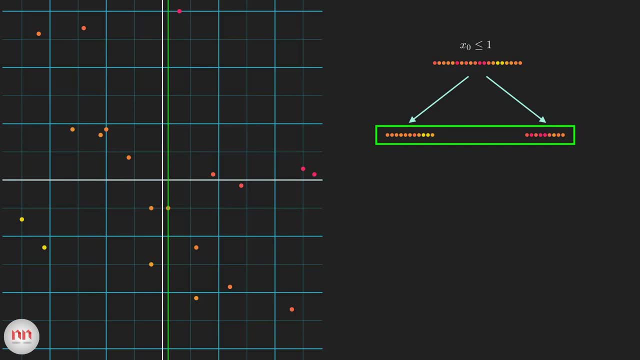 tree from scratch. If you liked this video, please share this video and don't forget to subscribe. Stay safe and thanks for watching. 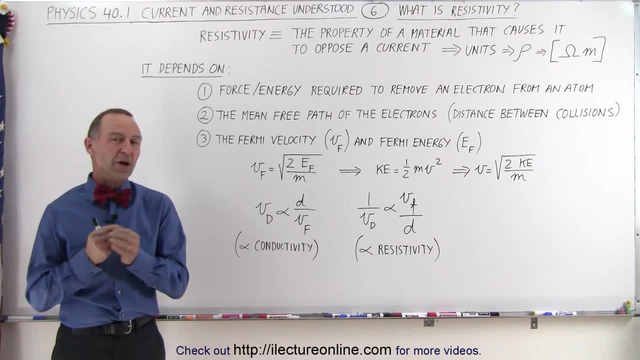 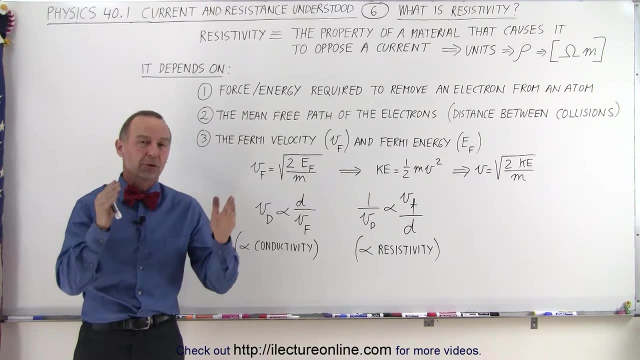 Welcome to ElectronLine. In the previous video we saw the concept of Ohm's law, where we saw that the current was proportional to the voltage applied and inversely proportional to the resistance in the circuit. But where does that resistance come from? Well, it's related to the 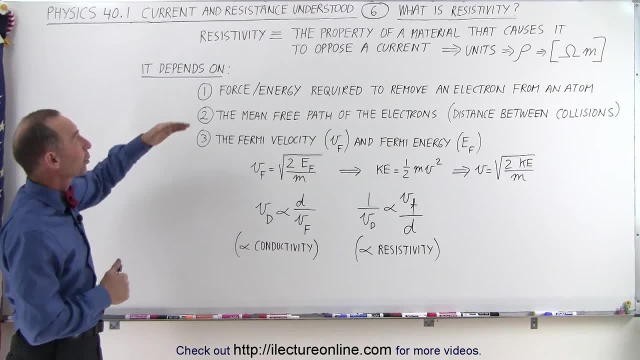 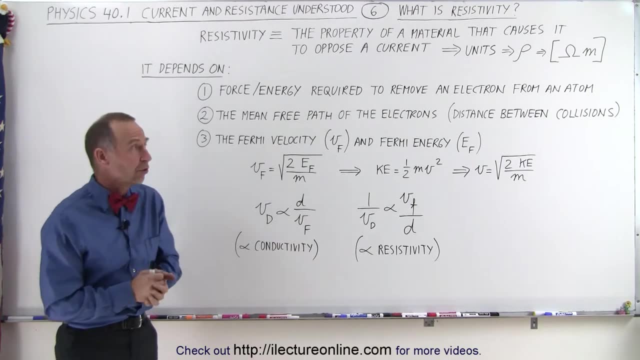 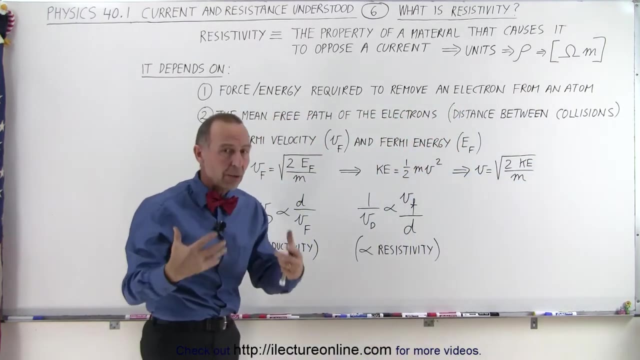 resistivity of the materials in the circuit. In other words, resistivity is the property of material that causes it to oppose a current, the flow of charges. We use the symbol rho for resistivity and the unit for that is ohms times meters, and later on we'll see how to manipulate resistivity. 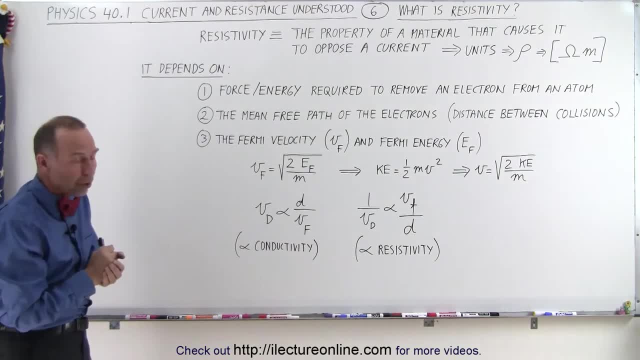 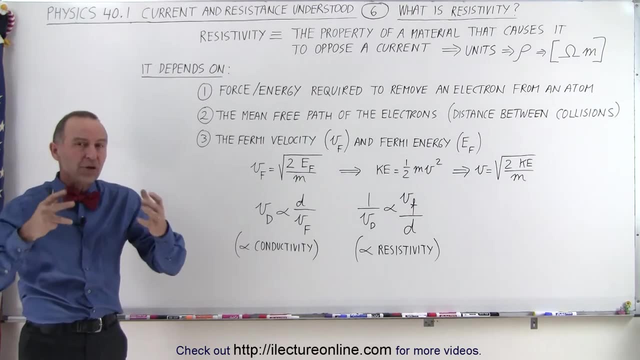 or how to find the resistance of an object once the resistivity is known and the geometry or the structure of the object is known. But the resistivity that property in a material that opposes the flow of charges depends on three main things. First of all, 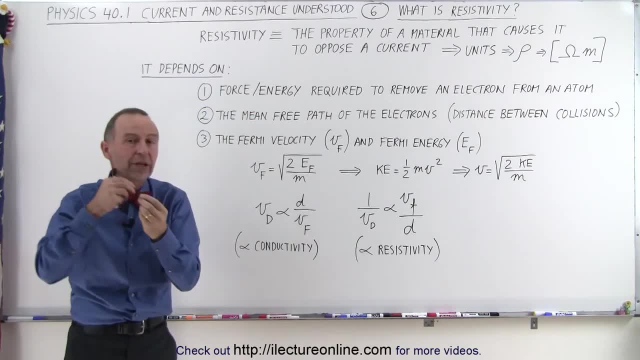 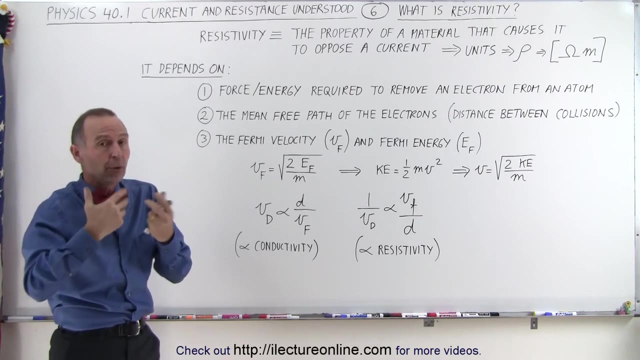 it depends on the force or the energy required to remove an electron from an atom. After all, for charges to flow, you have to have free charges and you have to be able to rip them away from the atoms inside the conductor material. And so how much energy and force that requires? Well the more.